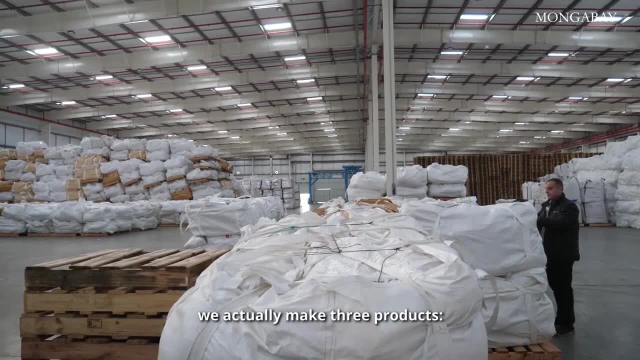 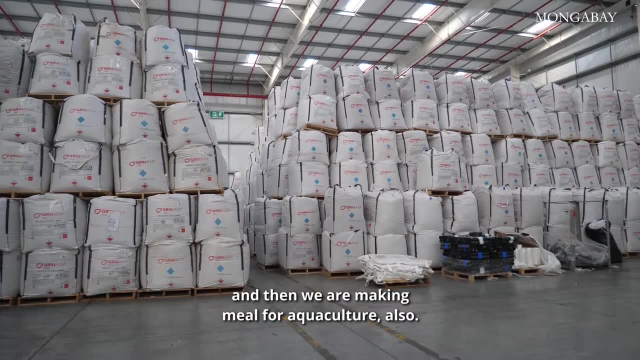 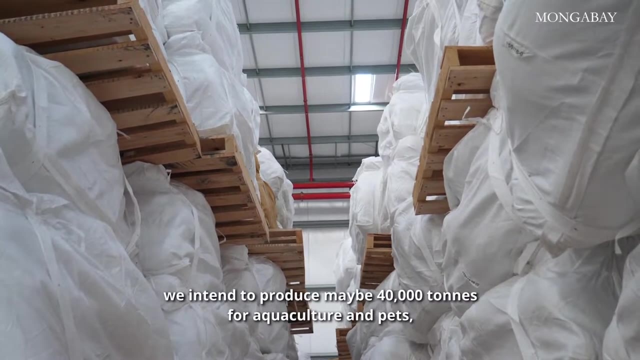 The krill is processed on board the vessels. We actually make three products: oil for human nutrition, meal for use in pet, and then we're making a meal for aquaculture also. Eighty percent of our volume goes to aquaculture We intend to produce. 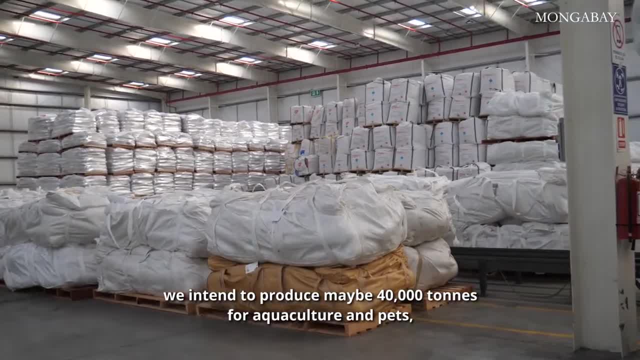 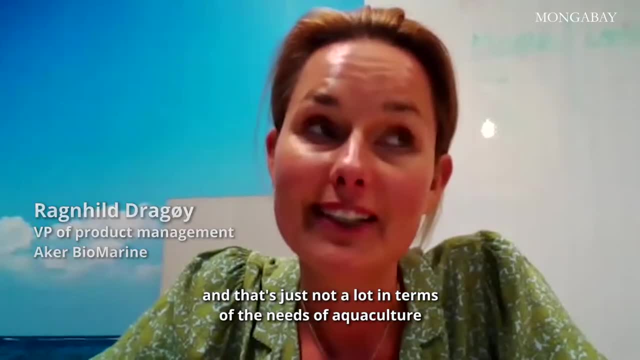 maybe 40,000 tons for aquaculture and pets and that's just not a lot in terms of like the needs of the needs of aquaculture, but it's one of those alternative ingredients that we're going to be using in the future. We're going to be using it in the future. 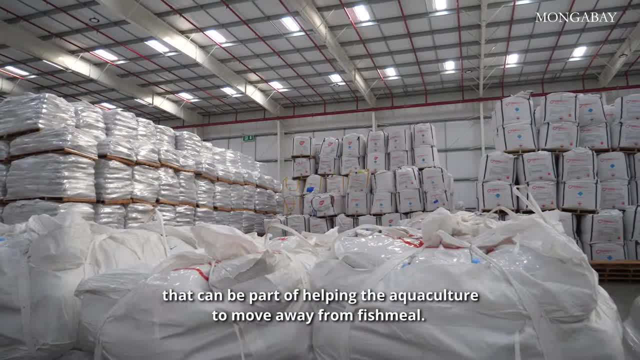 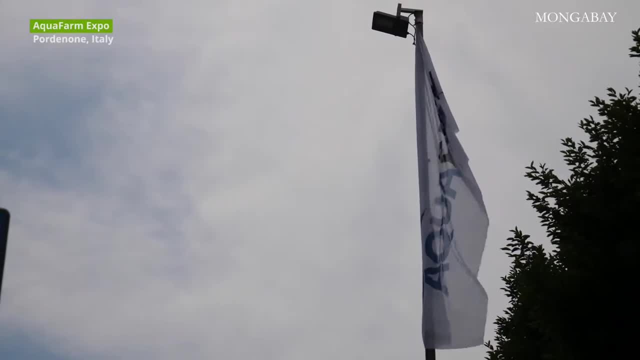 We're going to be using it in the future. We're going to be using it in the future. I can be part of helping the aquaculture move away from fish meal. There will be more and more different alternative materials for fish feed. 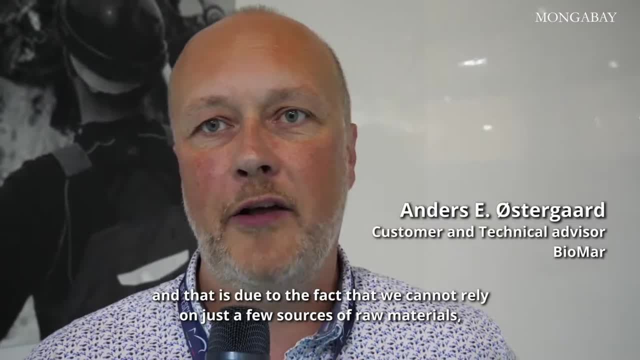 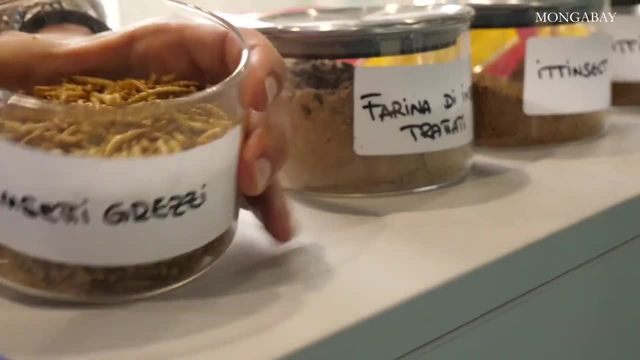 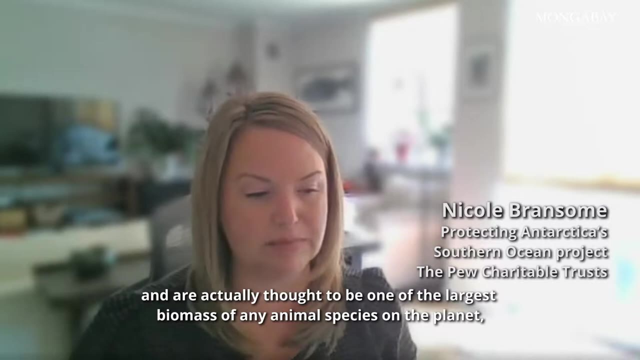 raw materials, and that is due to the fact that we cannot rely on just a few sources of raw materials, and especially marine resources, are scarce and limited. Krill, which form these massive swarms and are actually thought to be one of the largest biomass of any animal species on the planet. 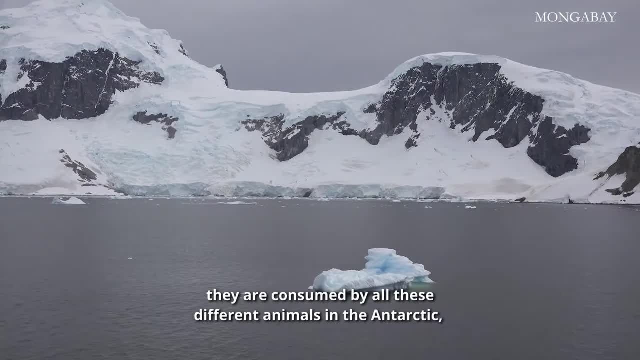 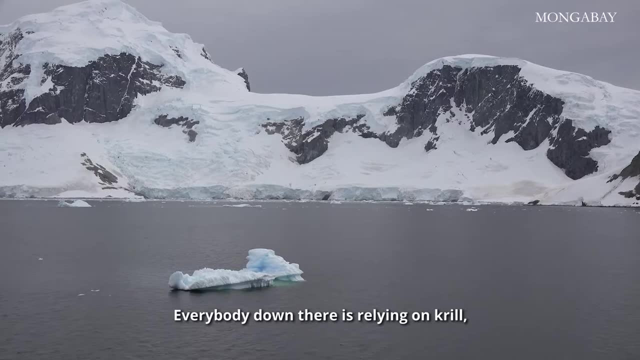 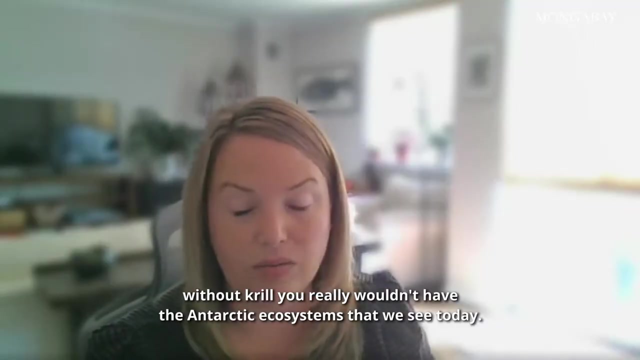 They are consumed by all these different animals in the Antarctic, from whales to seals, to fish, to penguins to flying seabirds. Everybody down there is relying on krill. Without krill, you really wouldn't have the Antarctic ecosystems that we see today. Exactly. We are allowed to catch only 1% of the total biomass available And this is very small amounts for our small pelagic species. Usually, for any anchovy or sardine fishery which produces fish meal, You are fishing about 40 to 60% of the stock. 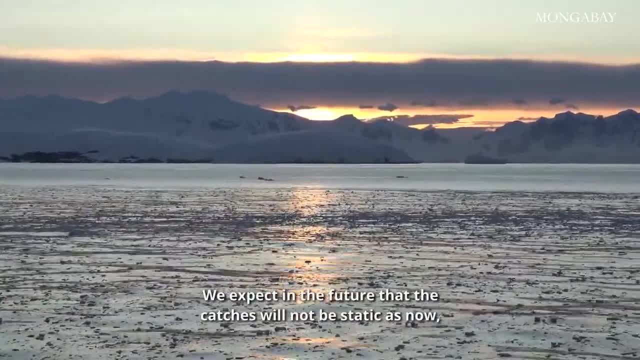 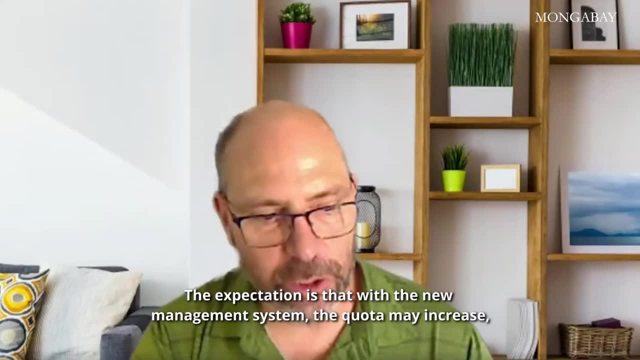 Here we are only fishing 1%. We expect in the future that the catches will be very high, will not be static as now. it will change year to year. The expectation is that with the new management system the quota may increase. I truly believe that it will increase. 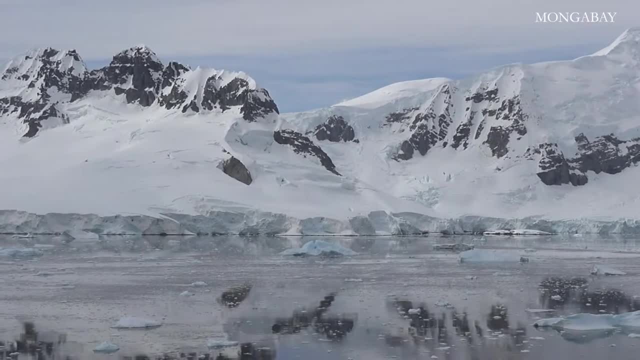 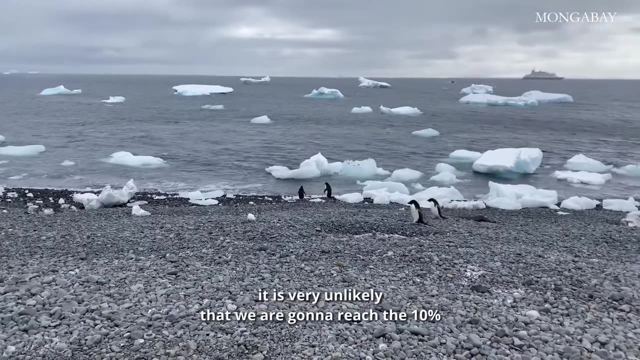 because, as I mentioned, the curse on the years is really abundant. All the numbers suggest that in order to keep healthy population of predators, it's very unlikely that we're gonna reach that 10%. I would venture that maybe just double that we have.